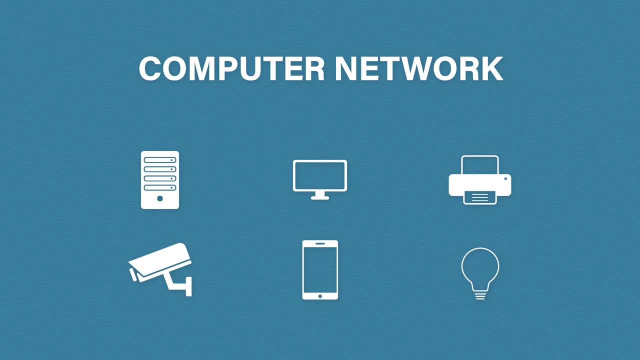 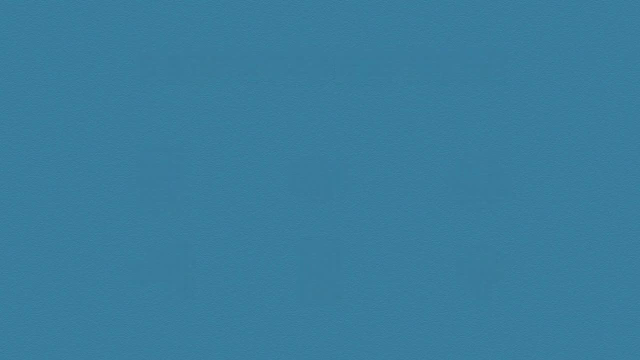 found on networks these days, And the list really does go on and on. So let's take a look at some basic networks and we can see what they look like. First one that should be familiar to most of you: Here we have a switch, a router, a wireless access. 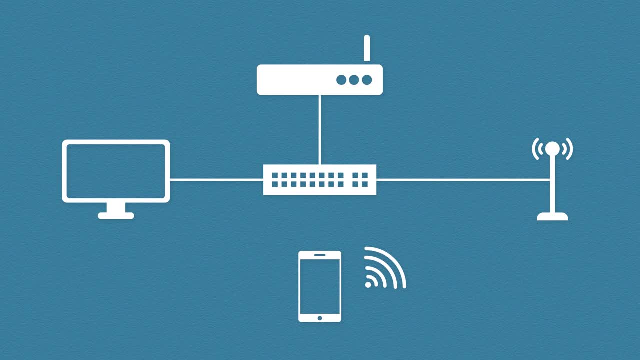 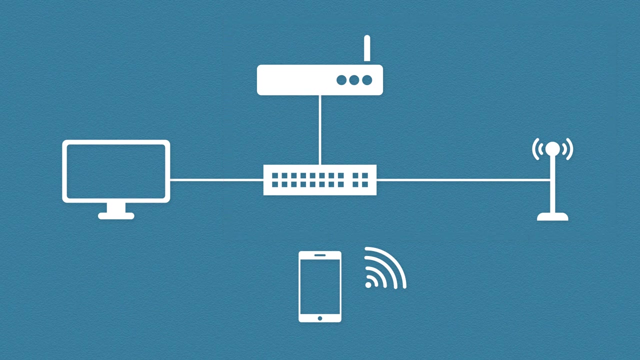 point a desktop and a phone all connected to the same network. This is a pretty common home setup. It's worth noting that in most home networks the switch and wireless access point will be built into the router. Generally speaking, any network in a single area is a system of connected people. 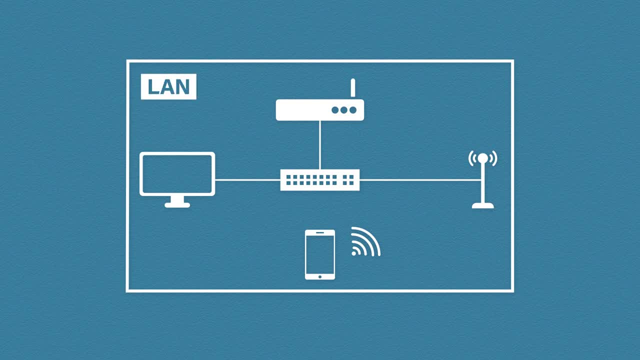 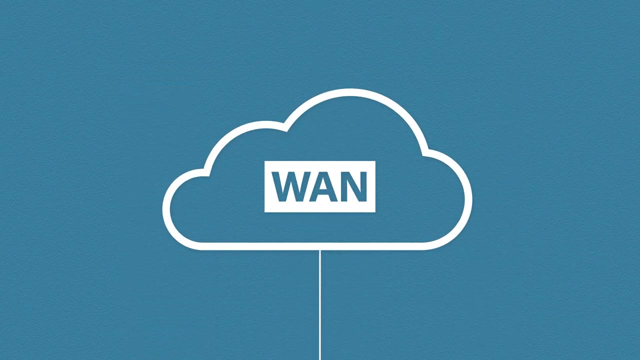 called a local area network, or LAN. The LAN is usually connected to the outside world using a socket in the wall that your internet service provider has installed. This socket connects you to something called the wide area network or WAN. The purpose of a WAN is to connect separate local area networks. 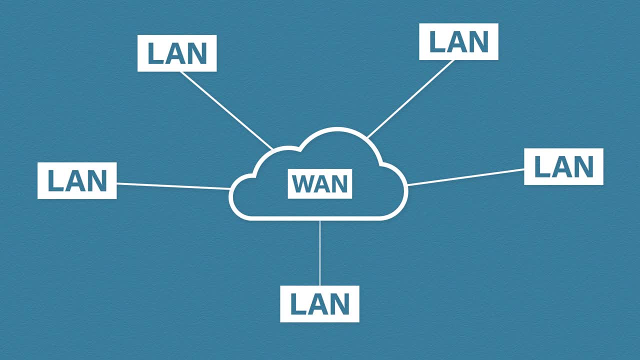 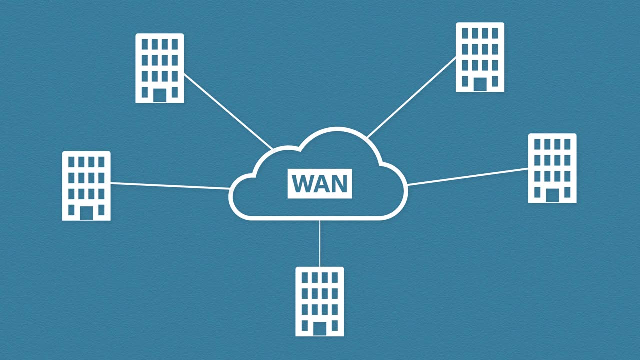 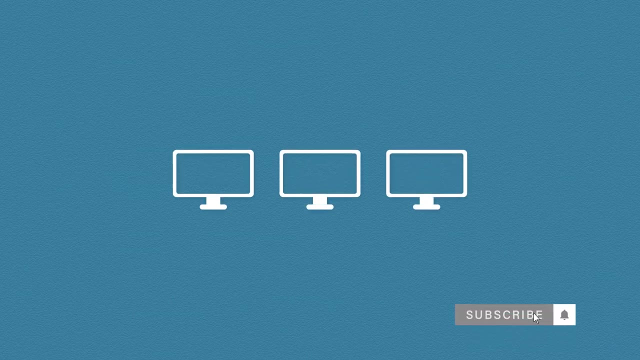 together. The most obvious example of a WAN would be the Internet. However, businesses might have private WANs to connect multiple sites together. So now let's look at a more business type network. So we have all of our office computers and these would usually plug into a wall or floor socket. These 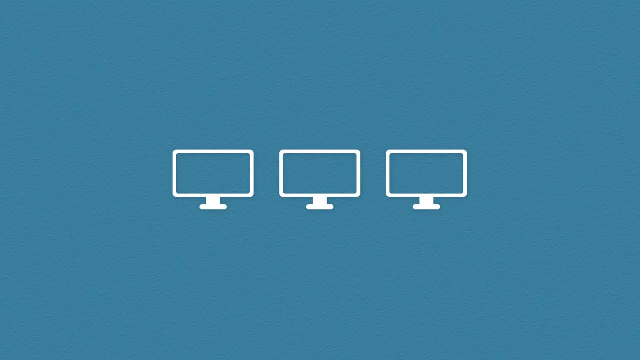 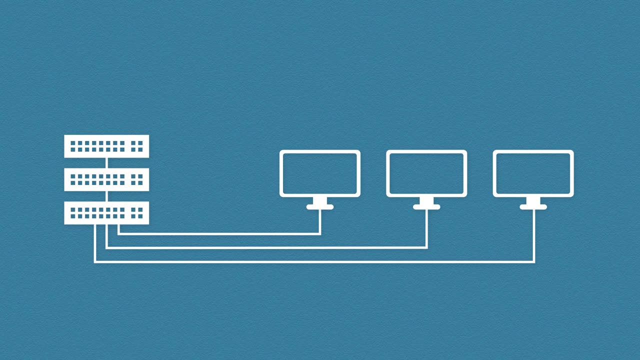 sockets will have cables either running through the floor or the ceiling back to a special room called a wiring closet. This room might also be called a patch room or a server room. In the wiring closet, all of these devices will connect to the internet. This is the most common way to connect to the internet. 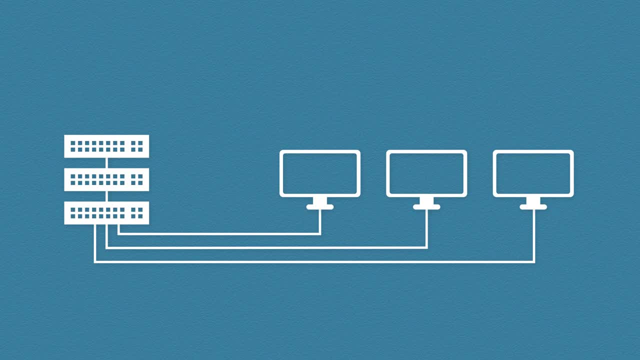 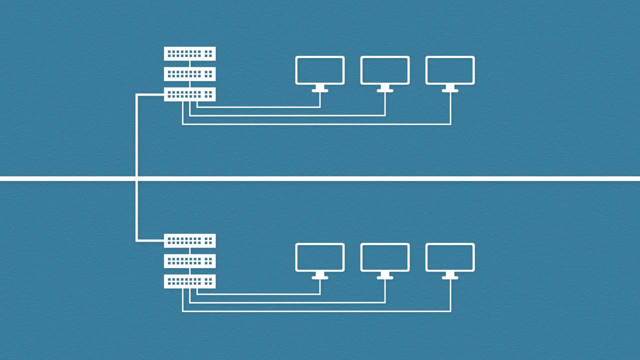 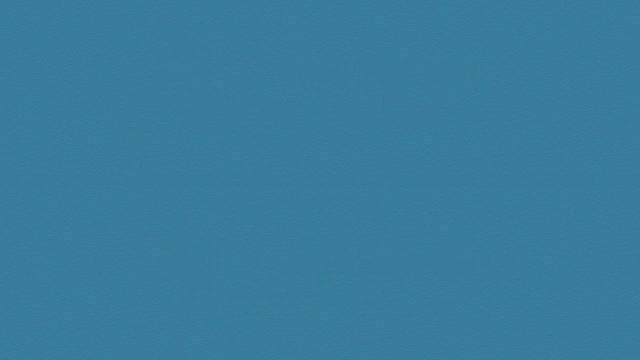 To connect to a stack of switches which are mounted onto racks. Depending on the size of the network, there may be multiple wiring closets which all connect to each other, Say, for example, on different floors. Keep in mind, though, this has been simplified to give you a general idea. Lastly, we'll look at 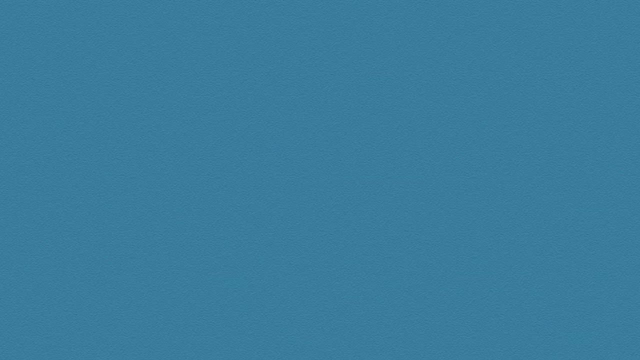 another type of network that might not be so obvious. Now, I said before, I'm sure you all have smartphones of some sort. Now these phones generally have internet access via 3G, 4G and even 5G. Well, you can think of these as. 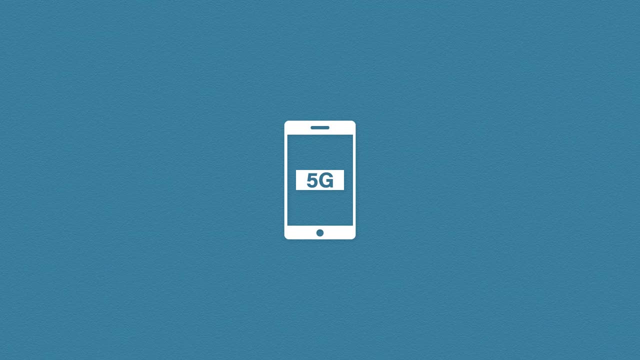 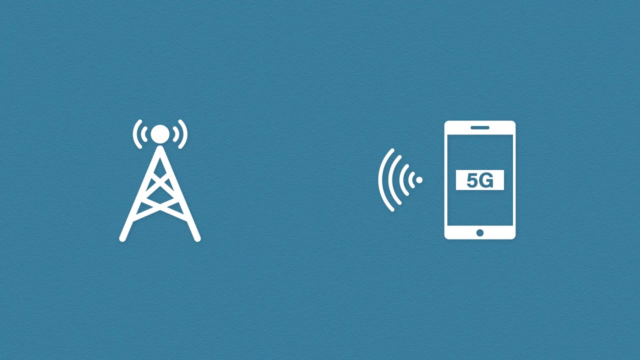 basically a giant wireless network for your phones. Somewhere close to you there will be a giant tower that allows you to connect and get internet access. The closer you are to these towers, the better the connection is likely to be. So these are just some common network. 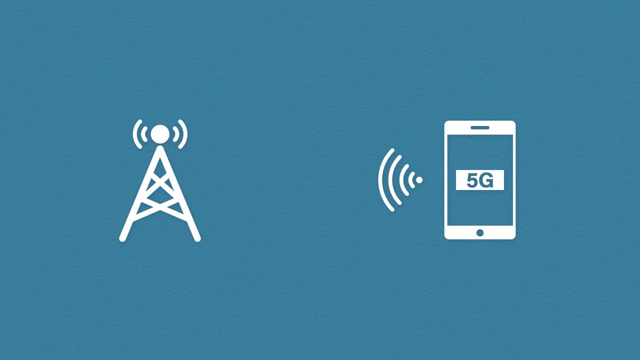 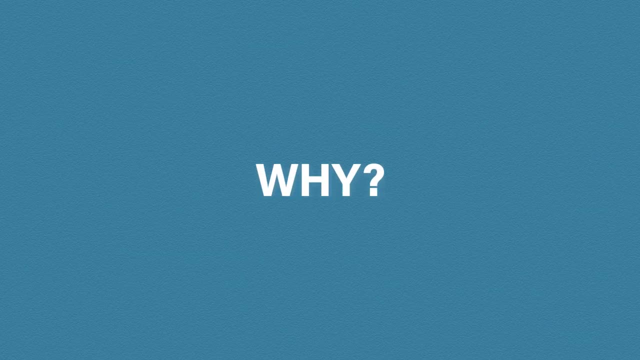 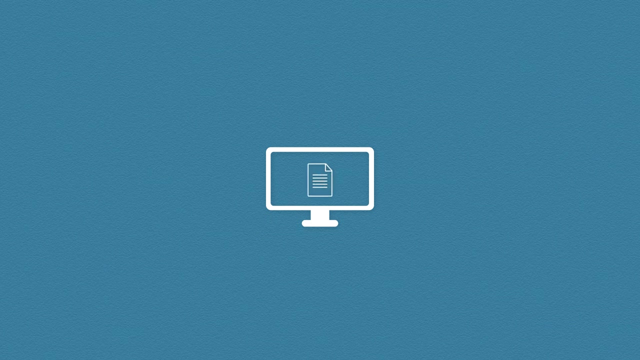 types and really just an introduction to some basic network devices. So the next, next logical question is: why? Why do we need networks? Well, let's imagine life without networks for a second. If we want to print a document, we would need to directly connect a. 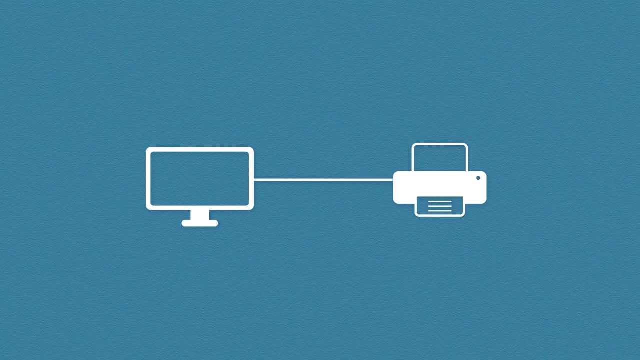 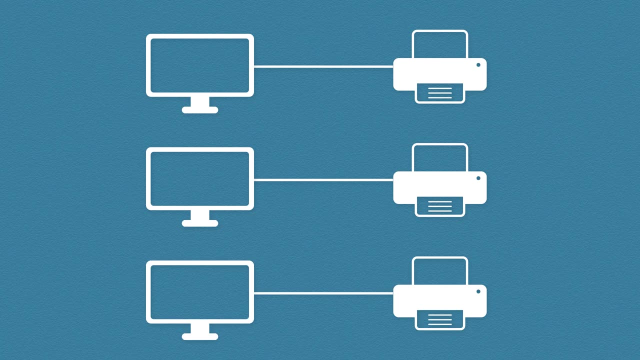 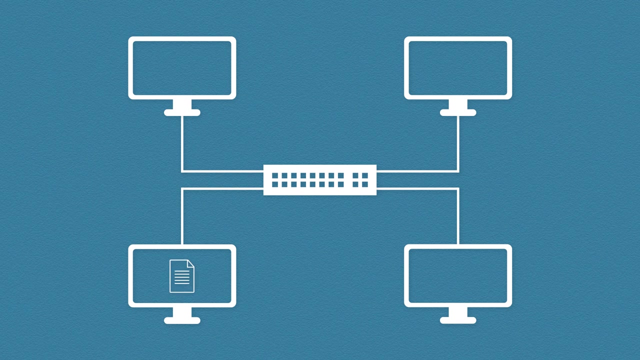 printer, which is fine. But what if we have multiple computers? We would need multiple directly connected printers, right, Which isn't so fine. The beauty of a network is we can share resources. If I have a file and I want to send it to someone, I can. They can also share the file with everyone. 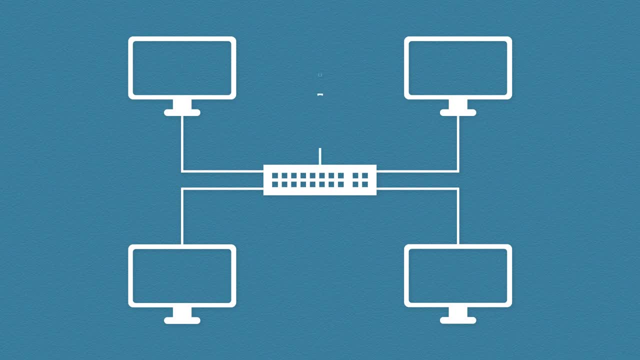 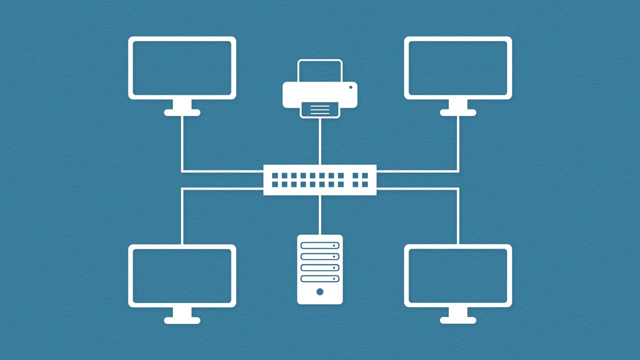 else. We can have shared printers that everyone can use. We can even have servers that could store these files for us. Of course, file sharing and printing is just one example, but this could be pretty much anything. And all of this even before we start talking about the internet, which, by the 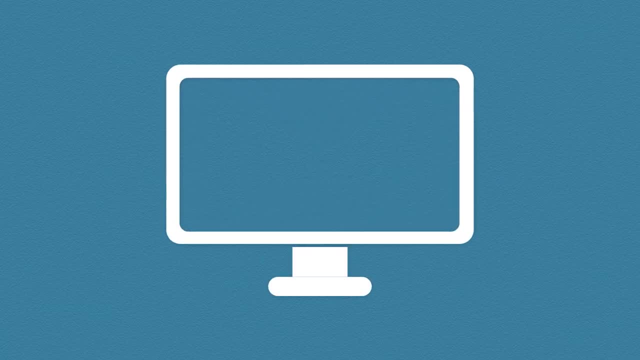 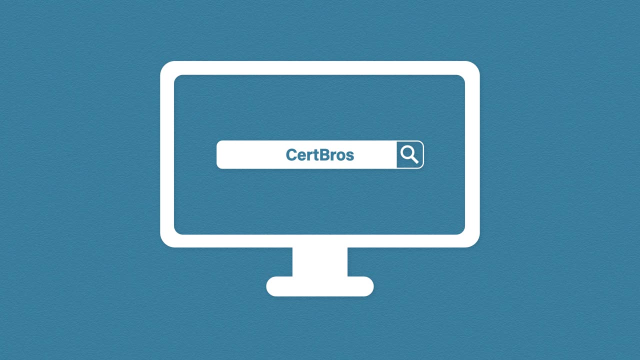 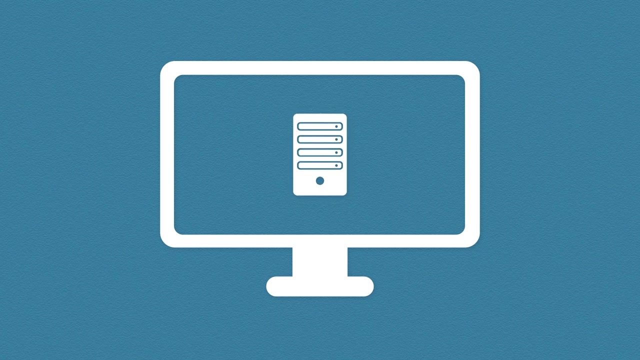 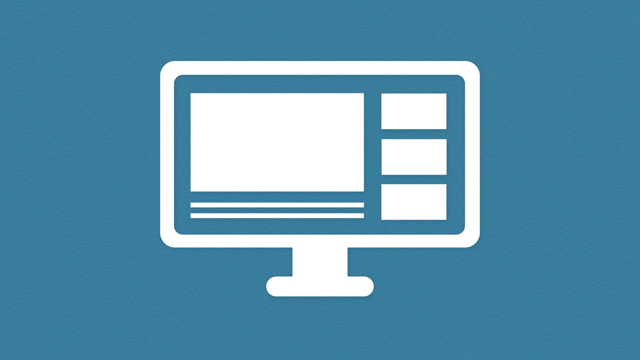 way is just a giant lie. Network With the internet we can search for anything we want. We literally have the world's knowledge at our fingertips. We have email, We can message our friends, We can use hosted computing, Telephone calls over the internet And, of course, awesome YouTube content. So networking has changed. 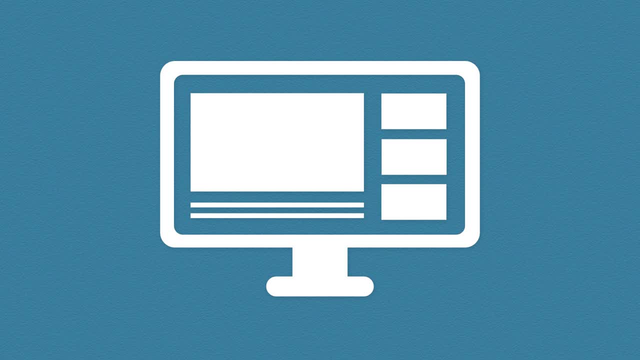 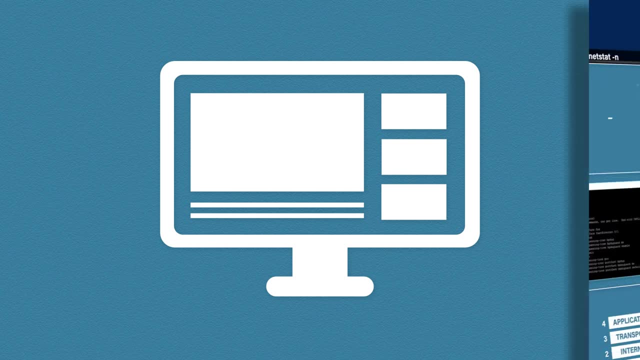 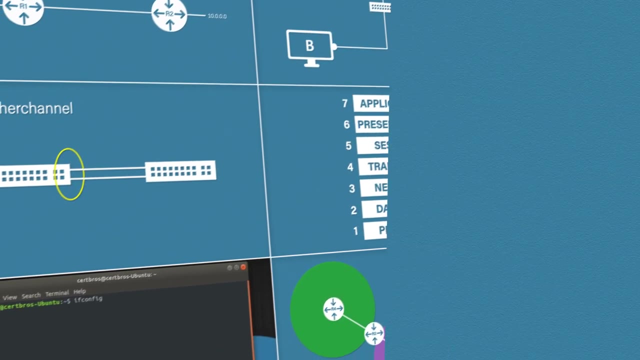 the world and how we live in it. It's a topic I still get excited about, and there's no shortage of things to learn. We'll go over a lot of this in more detail as we go. This video is part of our full CCNA course, which can be found in the description, So please feel free to go and check that out. 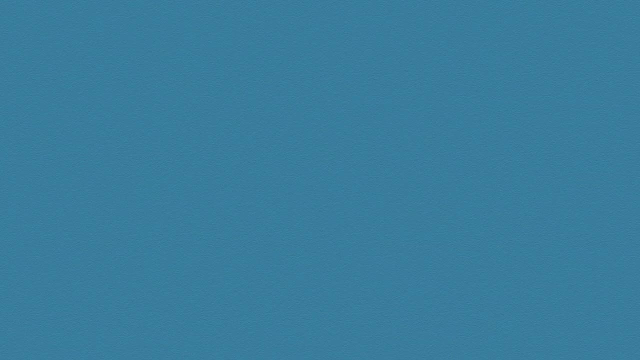 If you liked this video, don't forget to like, comment and subscribe. Other than that, thank you for watching. Subtitles by the Amaraorg community.